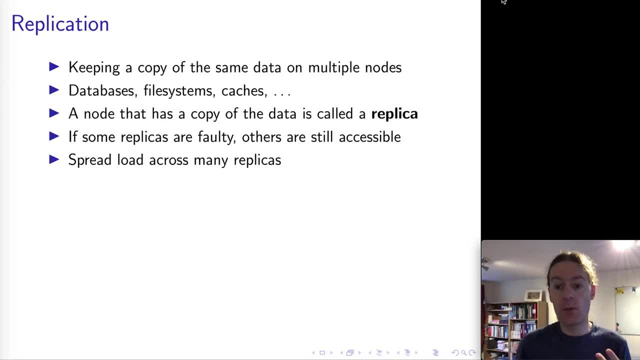 make nodes inaccessible from time to time. For example, you might choose to reboot a node in order to install software updates, And while that computer is rebooting it can't be processing any user requests or any messages, And so during that time that node is unavailable. And really what? 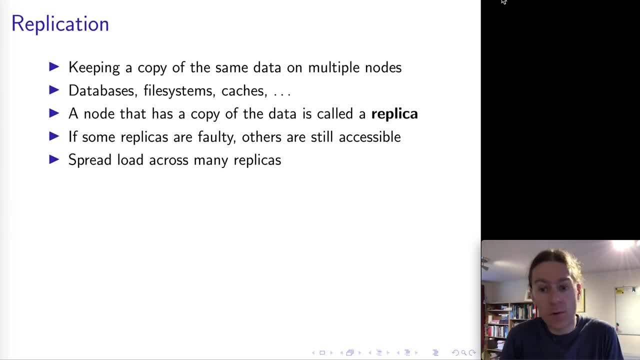 we want is that a service as a whole, of a database, for example. it continues working even if some of the nodes are unavailable, And replication is one of the mechanisms we have which allows us to provide that sort of fault tolerance, which is very useful, especially if you. 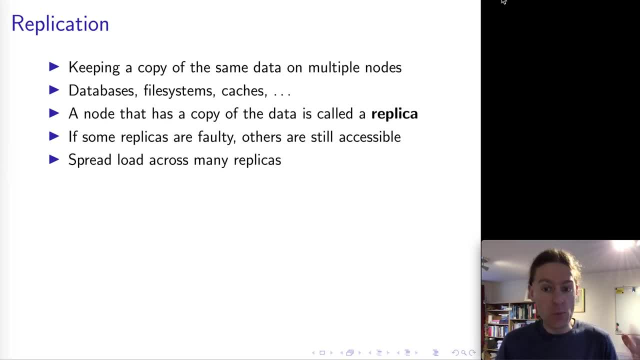 need to do maintenance of a system, because it means you can reboot one node at a time, as long as you're not turning them all off at the same time. as long as you just reboot one at a time, then the remaining nodes at any one time can continue processing requests- Another reason why 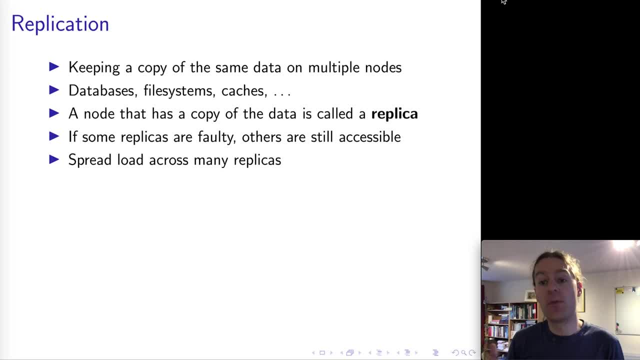 you might want replication is if there's very heavy load- for example, lots and lots of different users around the world all want the same piece of data- then that might be too much for a single node to handle, And in which case, having copies of that data on multiple nodes simply lets you handle more requests from more. 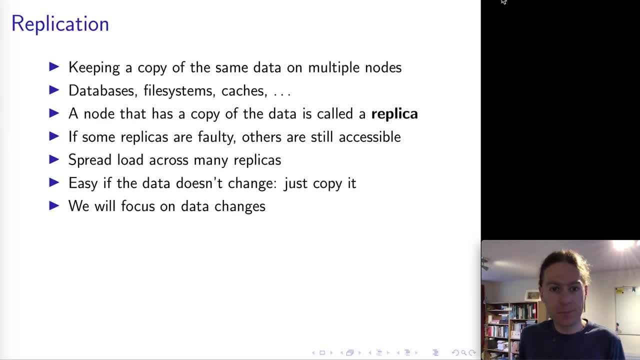 users, which is important in internet scale systems. Now, replication is really easy if the data that you're copying doesn't change. This is kind of obvious. If you've got some data that is static, you can just make a copy of it, a one time copy across all of your nodes. 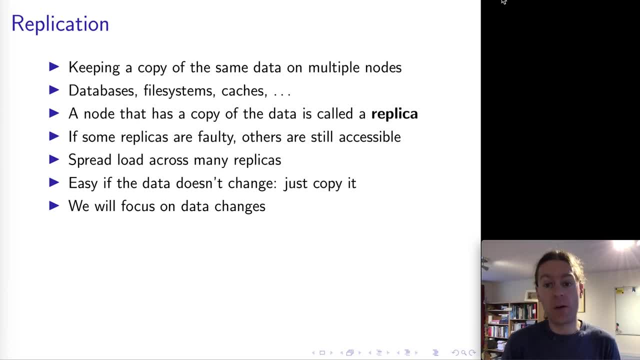 and then it's done. So what we're all going to be focusing on in this lecture is data that changes, because that's the bit that is hard. Data changes are the bit that is hard and that requires the most care. Now, one form of replication that you might have come across in the context of operating: 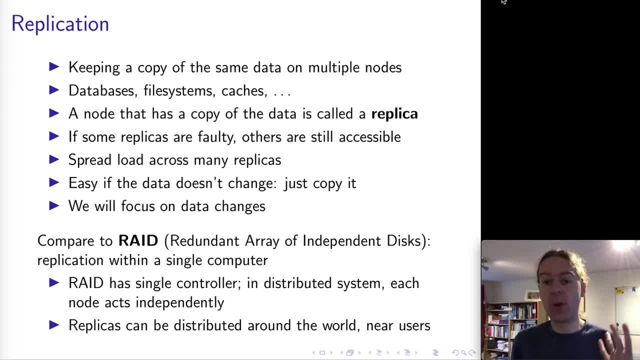 systems is called RAID, And so this is: if you have multiple hard disks attached to the same computer, you can use RAID to redundantly store data on more than one hard disk. So, for example, in the case of RAID, you can use RAID to store data on multiple hard disks. So, in the case of 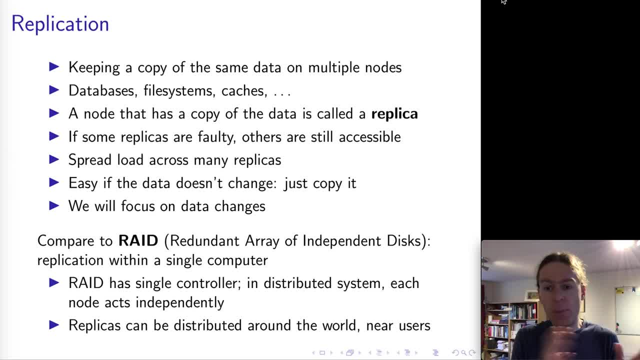 RAID. you can use RAID to store data on multiple hard disks. So, for example, in the case of RAID one, you actually have two separate disks that are basically mirrors of each other. So any file that is written to one disk is also written to the other disk, which means that if one of those 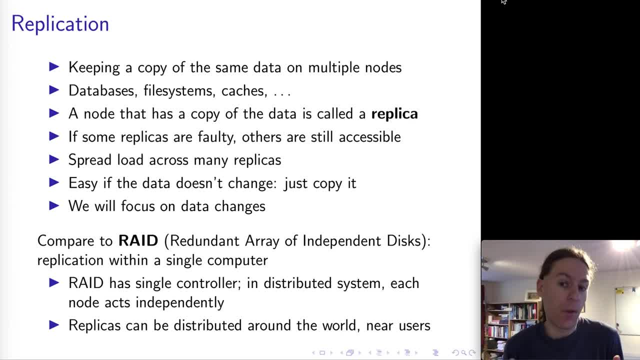 disks experiences a hardware failure, you've still got the data on the other disk- Extremely useful if you don't like losing data. Now, the replication that we talk about in distributed systems is somewhat similar to that, except the techniques that are used for RAID don't immediately apply. 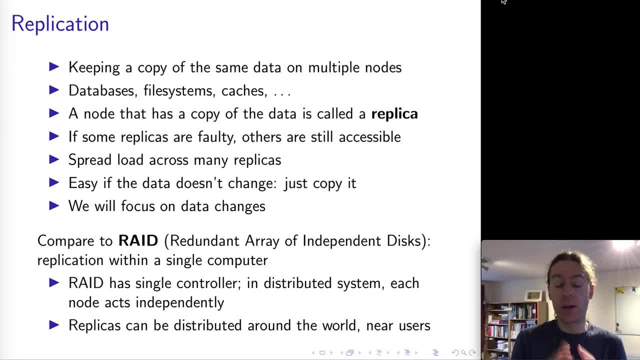 in a distributed system because RAID is designed for a single computer. there's a single controller that manages all of the data. In a distributed system, as we've seen in the previous lectures, we've got each node acting independently. we've got the unreliable network in between the two nodes. the nodes might be distributed around. 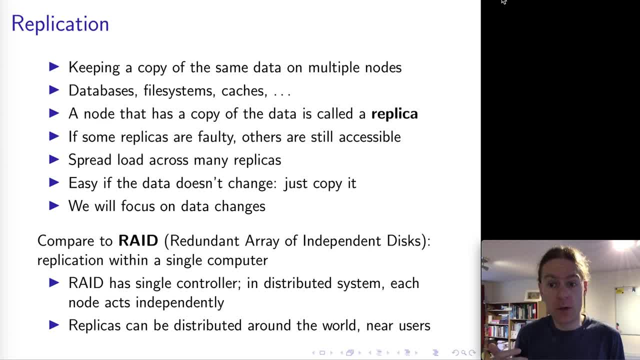 the world, so they might be not located in the same location, but they might be on different continents, communicating over the internet, And so we have to deal with all of the challenges that this sort of distributed setup brings. So let's look at one example, just to get us started. 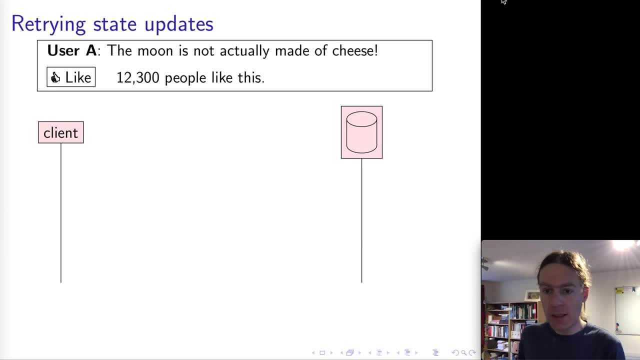 We've got a database that is storing some state and that state changes. So here we have an example of a social network and some user posts an update saying the moon is not actually made of cheese, and you want to press the like button on that. Okay, so the fact that you have pressed that like 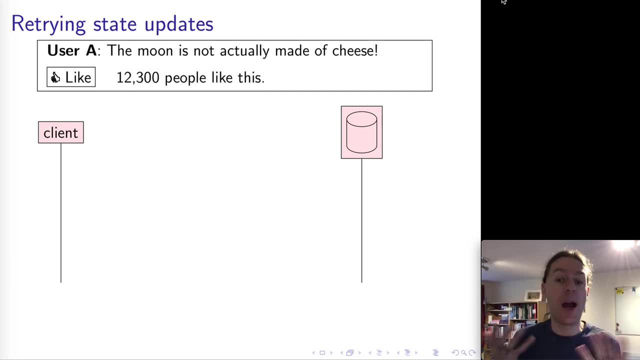 button needs to be stored somewhere, And also the fact of how many people have clicked that like button needs to be stored somewhere, And that somewhere is typically a database that is running somewhere on the servers of the social media provider. And what could happen now? 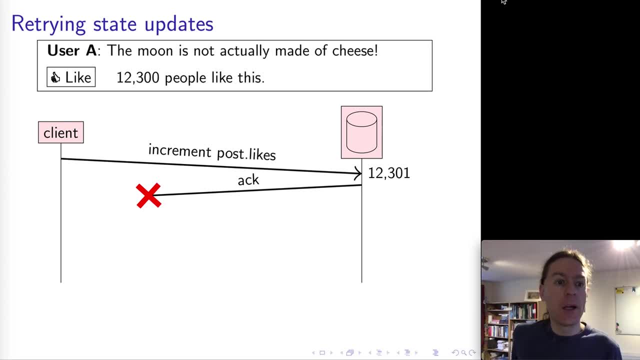 is. I'm just going to consider the count of likes for now. So the client, just as you press the like button, the client needs to tell this counter that is stored somewhere that, oh, you need to increment the counter because one more person has liked this particular update. now. But networks. 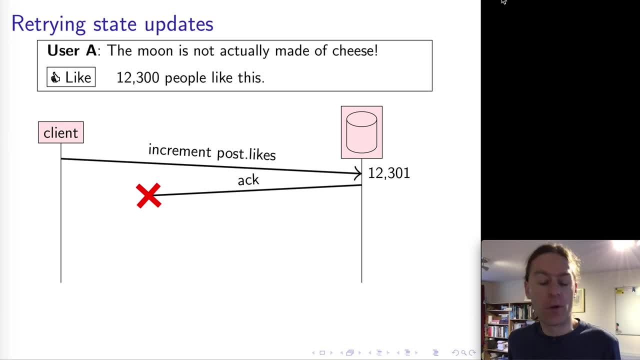 being what they are. of course, it could happen that either the request or the response is lost in the network. And so let's consider that, And so let's consider that, And so let's consider in this example that the request got through, but the acknowledgement back to the client that 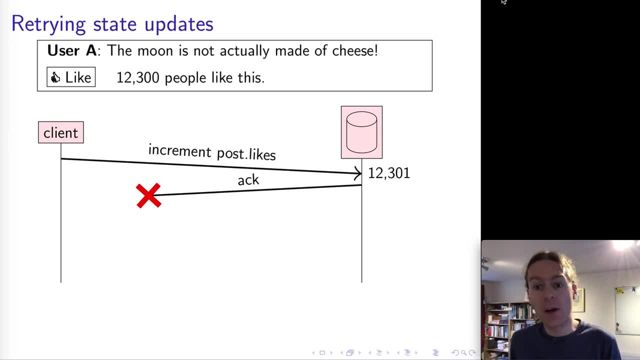 okay, I incremented the counter. The acknowledgement got lost in the network, And so the client says: well, it seems like the request didn't get through. Let's try it again. Let's send the request to increment again. The server receives that request again, And so it. 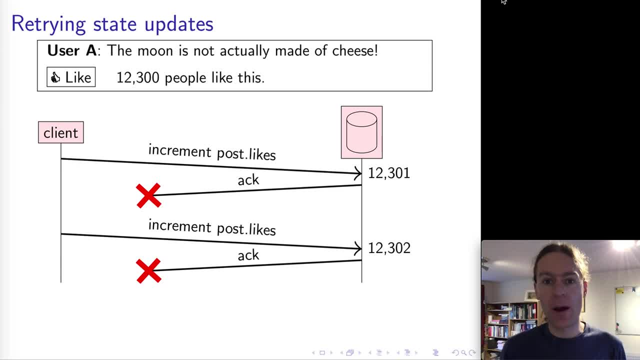 ends up incrementing this counter twice, And so we go from 12,300 to 12,302, even though you actually only pressed that button once. Now, this might seem like a bit of a hypothetical example, but it really does occur. Now the first. 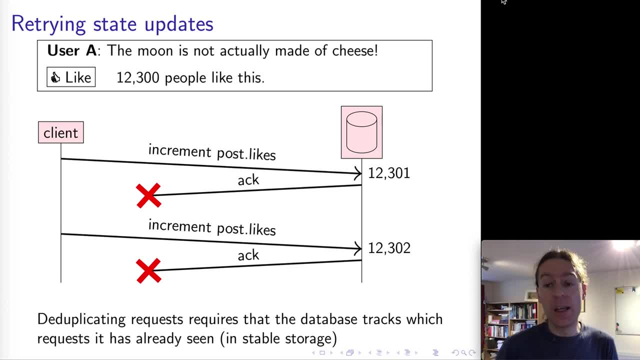 thing we can do to try and prevent this kind of thing is to do deduplication, And we've seen that in the context of the broadcast protocols, for example. However, with databases, with a database generally, we want to support a crash recovery type system model. That means you know if a 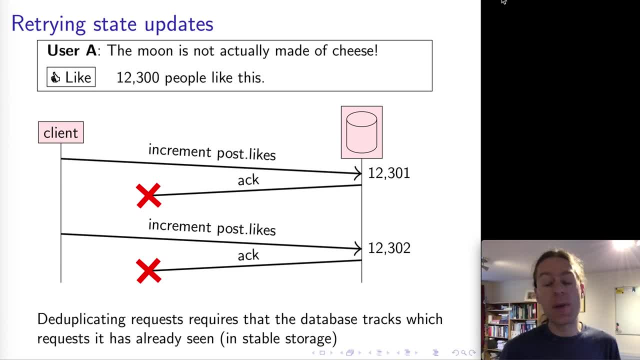 node crashes, it doesn't stay offline forever. It will come back, which is a very, very important thing, And that means that any data that needs to be not lost in the process of that crash and restart needs to be stored on disk in stable storage in some durable form And, if you want, 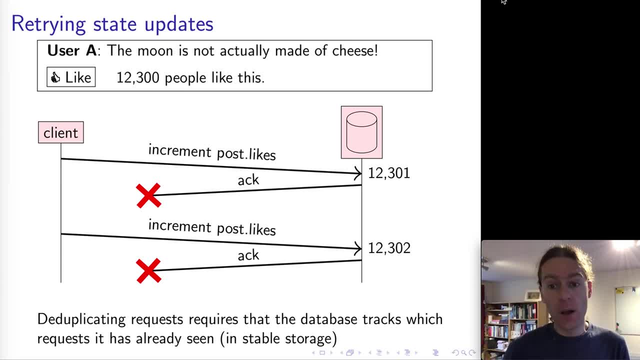 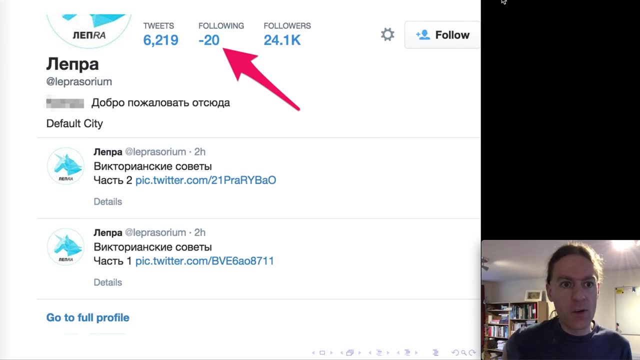 to deduplicate requests to a database in a way that will work even across crashes and restarts. that means that all of the requests actually need to be stored in the database as well. That can end up being quite a lot of data. Now you might think that this sort of thing is just 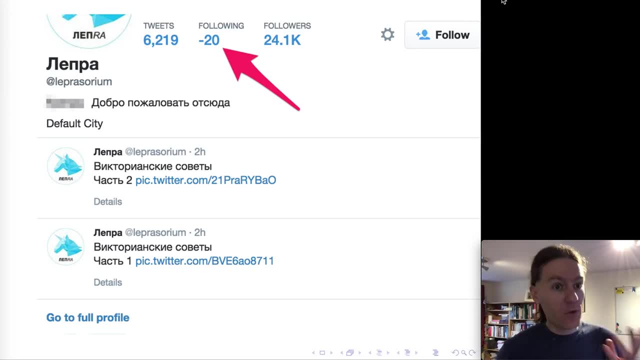 it really does occur. This is an example. This is a screenshot, a genuine screenshot- that I made of Twitter a few years ago, And it shows a user account who is following minus 20 people. So this should be impossible, because, of course, you can only follow a positive number of people. 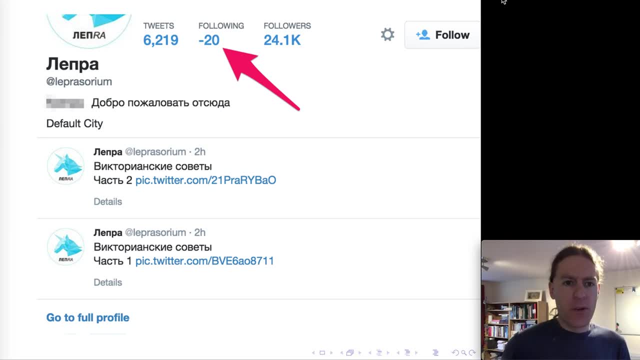 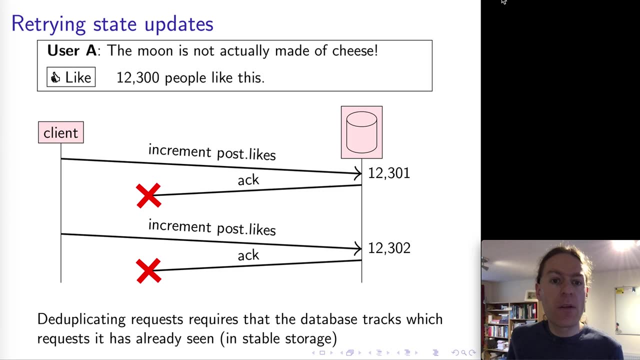 in real life There are no negative users, And so I don't know exactly what happened in this, in this scenario here, but I suspect that something happened, was very similar to the example, So probably the user was following some number of people, Then they unfollowed those. 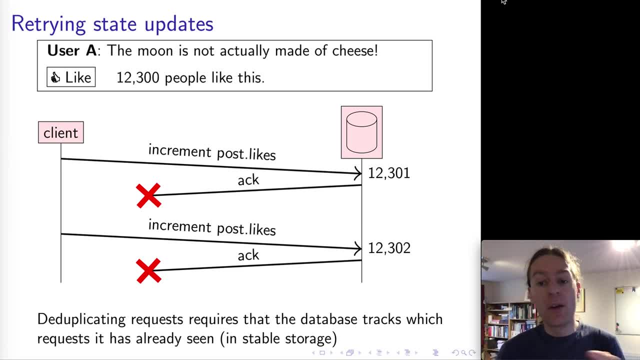 people in the process of unfollowing those people, Some counter of how many people this person is following had to get decremented, And so there was some network failure somewhere, And so that decrementing of the unfollow count- sorry, the decrementing of that follow count. 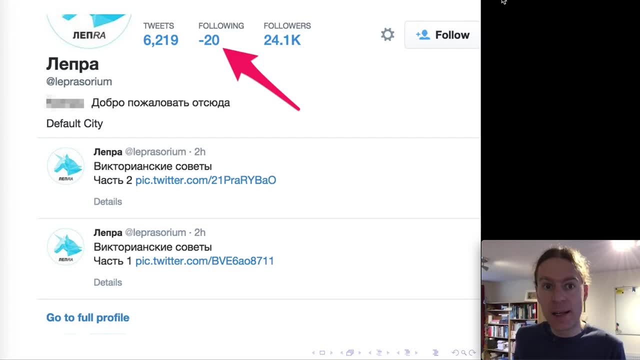 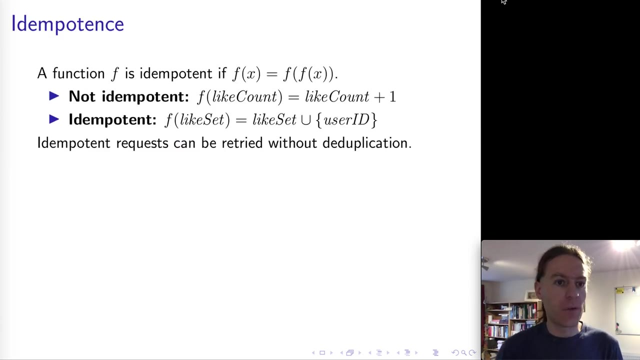 got repeated, And so we end up decrementing more than there were actually followers, And so that's why we end up with a negative counter here. So, OK, I think Twitter has probably fixed that bug in the meantime, But let's look at how we would deal with this kind of problem in our systems And 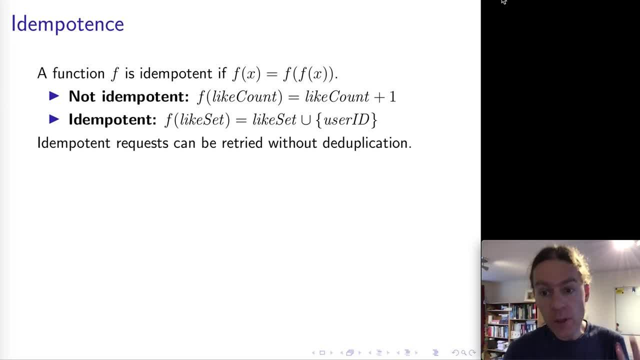 one tool that is very useful in the context of these kinds of retries is to make the operation idempotent. So idempotence is a concept from maths, which just means that if you apply a function once to some argument, it has the same effect as applying it. 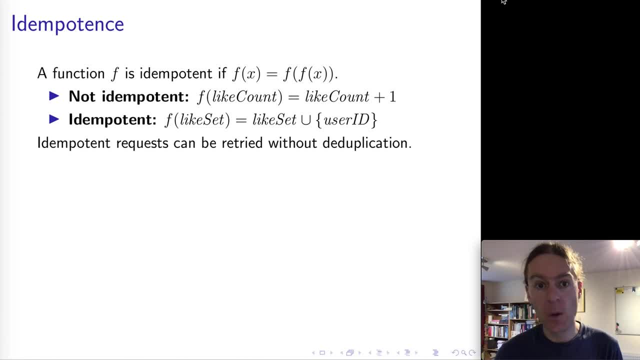 Twice, or applying it three times, or applying it any number of times, And so an example of a function that is not idempotent is to increment a counter like we have just seen, because if you increment a counter once, that's not the same as incrementing it twice. However, adding an element to a set is 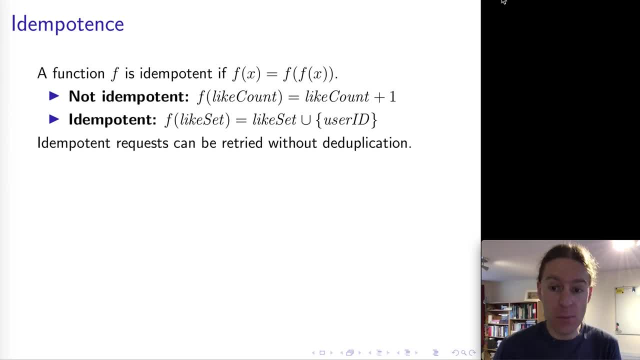 idempotent because if you add an element to a set and then add the same element to the set again, because the set doesn't count how many times an element is there, it's either there or not there And so therefore, doing the set union operator, that is idempotent. 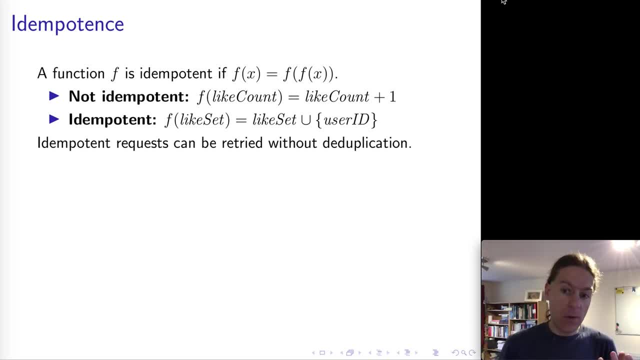 And so this means now, if we represent these likes or the user follows in the case of Twitter as a set rather than as a counter, then we can safely retry, because even if the request gets lost, or so we can just send that request to add an element to a set, We can do that again. 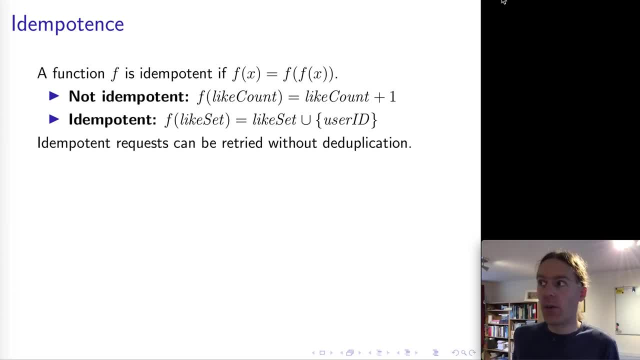 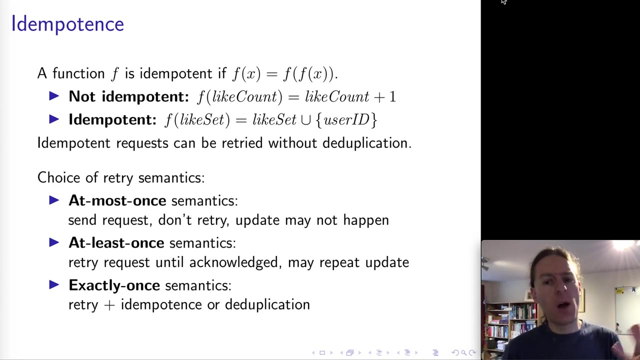 and applying it twice does no harm, because it just does the same as applying it once, Which leads to a choice of a set Of different semantics that you get in these types of distributed systems. they're just terms that you might see, and so I wanted to mention them briefly. 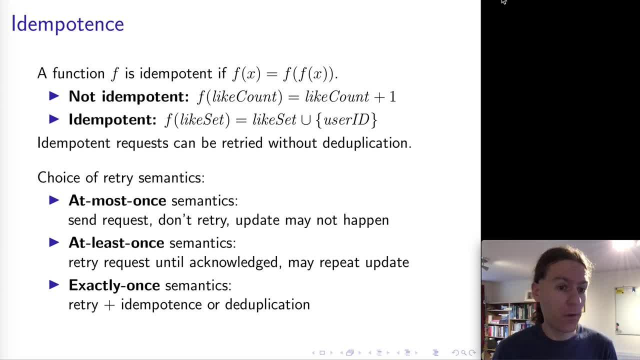 which are at most once, at least once and exactly once. So at most once just means you send a request over the network once. it may or may not get there, but you're not going to retry So it might arrive. it might not arrive, but you're not going to try and make this reliable. 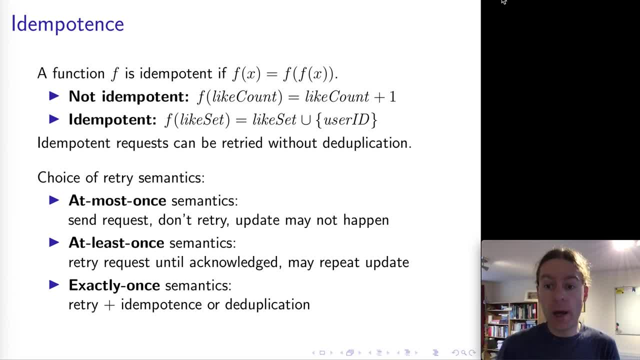 in any way. At least once means that you're not going to retry. So at least once means that you're going to retry until you get an acknowledgement, which means the request may arrive multiple times, but really what we typically want is exactly once, which means the operation. 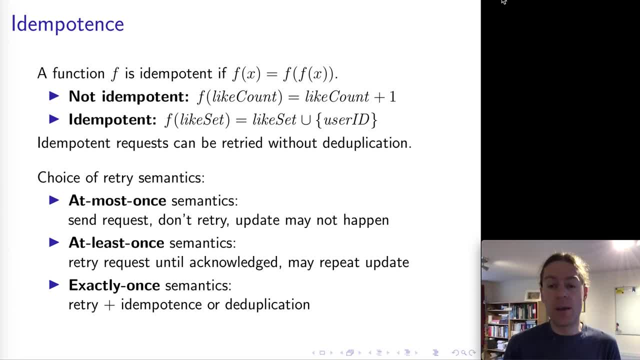 takes effect exactly once. So the effect is as if the operation were received exactly one time, even though in practice, due to retries and due to message loss, it may actually be some different number of times, And so if we retry and also again send could be several times pretty common, because 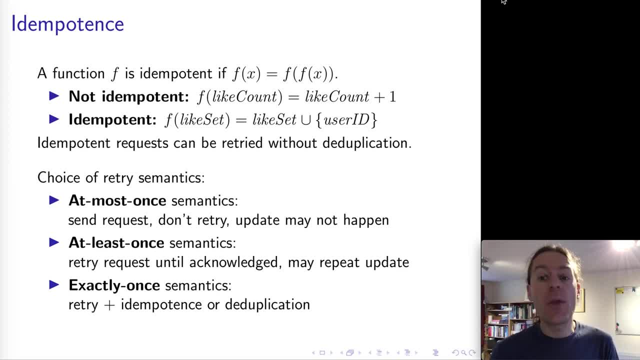 have an operation that is idempotent, then we can achieve exactly one semantics. So that means, even if the operation is applied multiple times, the effect is as if it had been applied exactly once. Or, of course, we can achieve exactly once through deduplication as well, as long as we're. 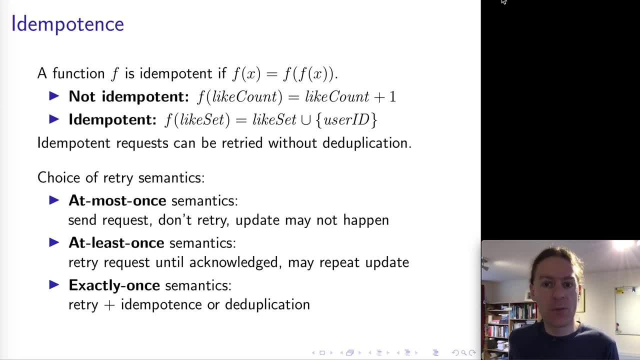 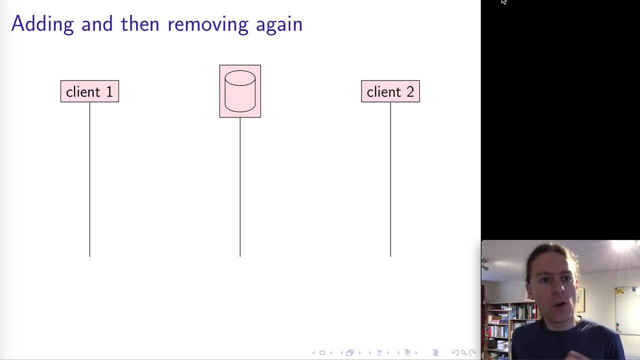 willing to store the requests that have already happened in some form. So let's have another problem. look at another problem which highlights the limitations of idempotence, And that is we've got two different clients this time, And client one wants to add a like or add your user ID to. 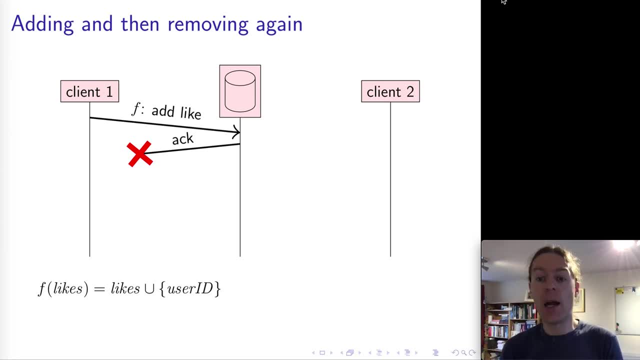 the set of users who have liked a particular update. And, as we've seen, this is an idempotent operation. this function f is idempotent. Now, client two reads from the database. it reads the current set of users who have liked it and it reads the current set of users who have liked it. 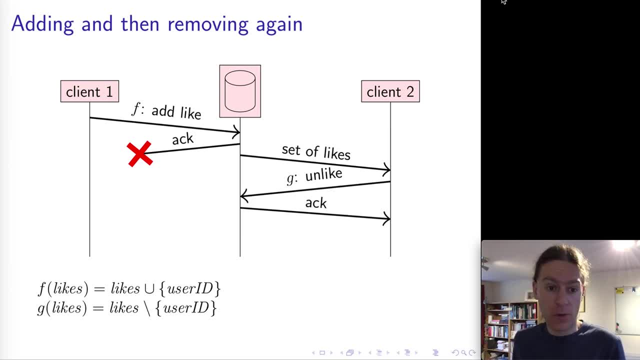 And decides to unlike this, And so what this means is to remove a particular user ID from the set of users who have liked a particular update, And client two makes this request g and sends it to the server, and the server acknowledges it. Now, the first request that client one made. 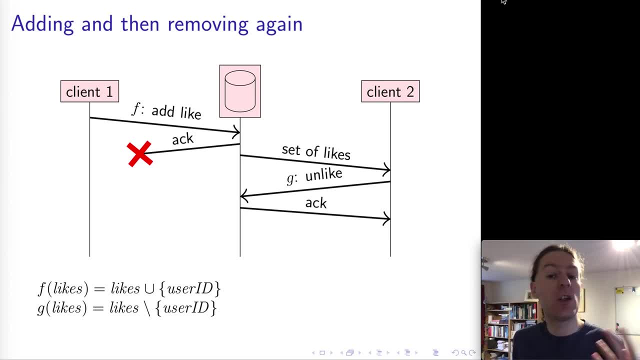 the acknowledgement got lost in the network, And so client one is going to retry this request, And so what the effect is now is that client one sends this request to add the like back to the server again, And the server, though, has actually just 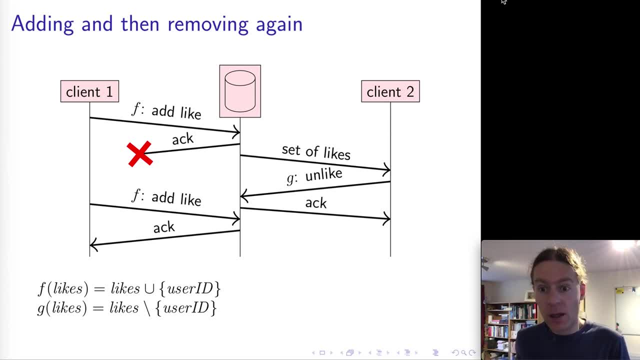 removed the like from the set of user IDs And so it's going to add it back in again. And so here, even though the function f is idempotent, so applying the like twice has the same effect as applying it once, in the context of also having this unlike operation, actually the idempotence. 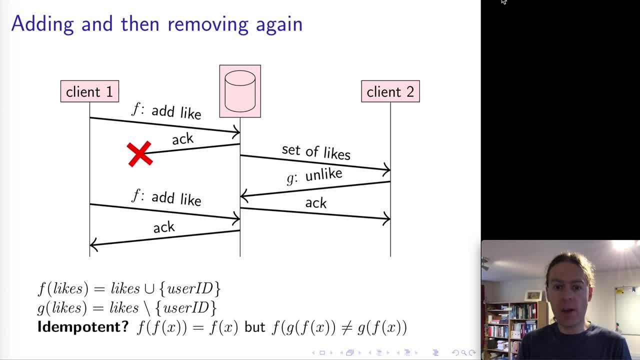 doesn't quite work anymore, Because if we apply first f, then g, then f, then this is not the same as just applying first f then g, because the second application of f is going to add the element back into the set again, And so here the user intention was that. 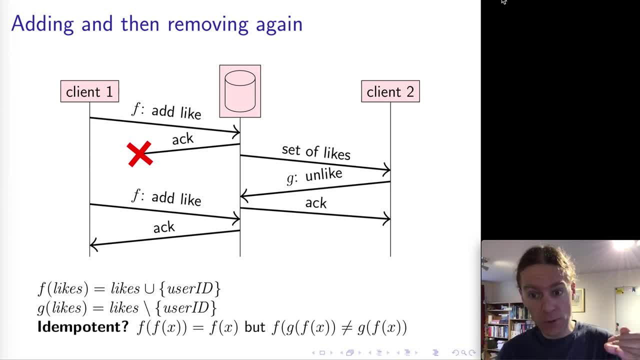 this item should not be liked, because the user first liked it and then unliked it And this retry of adding the like still causally belongs to this first request here. So it's not a separate request to add it back in again, But the actual intention. 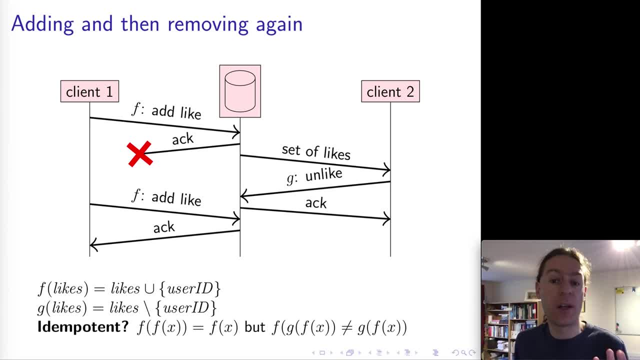 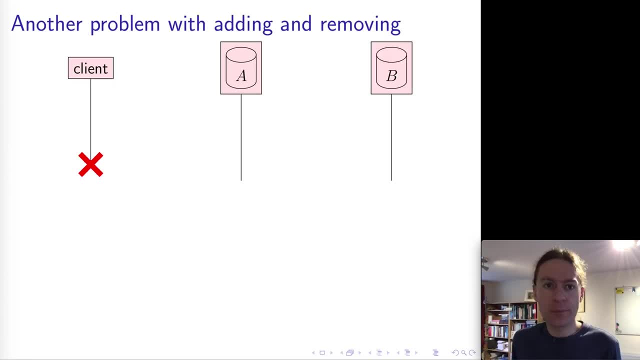 is to add the element back into the set again, And so here the user intention was that this item is not liked. So let's have a look at an approach that we can use to solve this problem, And I will illustrate this with another problem that can happen with replication, And so in this, 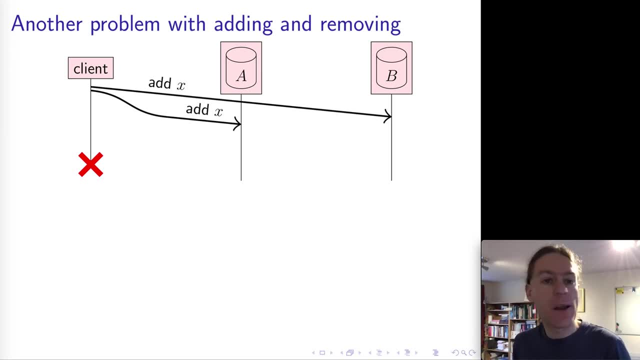 case. here, what we have is a client that wants to add an element x to a set, So I'm just going to treat it more abstractly- Let's forget about status updates and likes for now- And just more abstractly, we have some element x that needs to be added to a set, And so we're going to 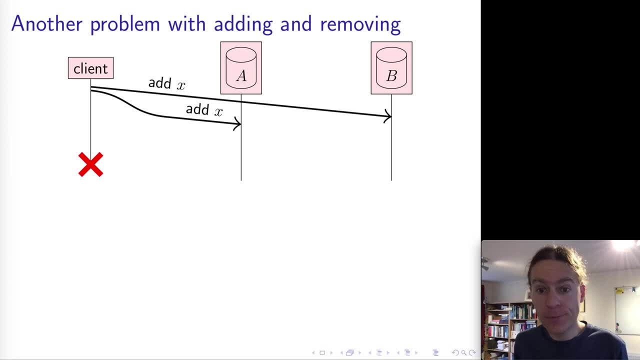 have a set on both replica A and replica B And first the user adds it And then the user wants to remove it again because people can change their minds. Okay, fine, And so first we have an add request that goes to both replicas, Then we have a remove request. Now, unfortunately, 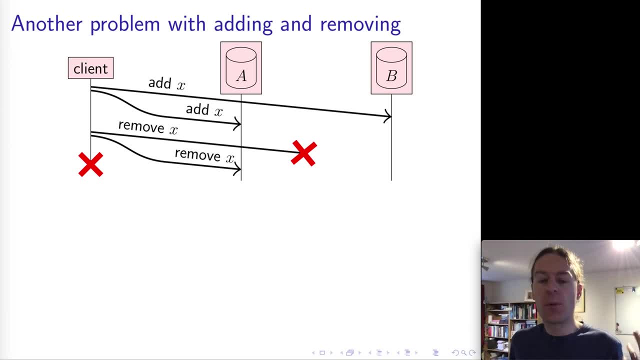 the remove request is lost in the network on its way from the client to replica B. So replica A receives both the add and the remove, But replica B only receives the add, doesn't receive the remove. So the end result now is that the element x is in the set on replica B. 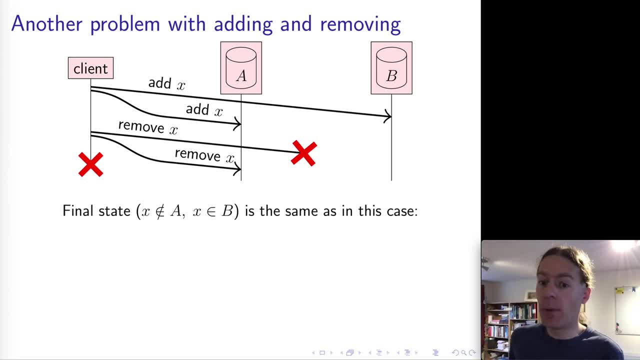 because it hasn't been removed, But x is not in the set on replica A because it has been removed. Now, if you think about this, the state of the two replicas in this example here is exactly the same as in this example. So in the second example the client wants to add x to the set. The addition: 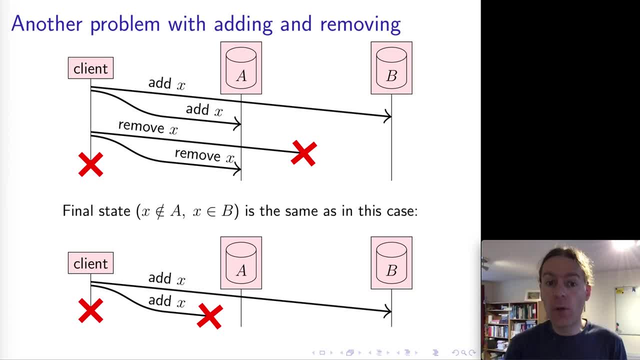 goes through and reaches replica B, But the addition is lost on its way to replica A. So again we have the same state, that x is present on B but absent on A, So that the final state of the two replicas is the same in these. 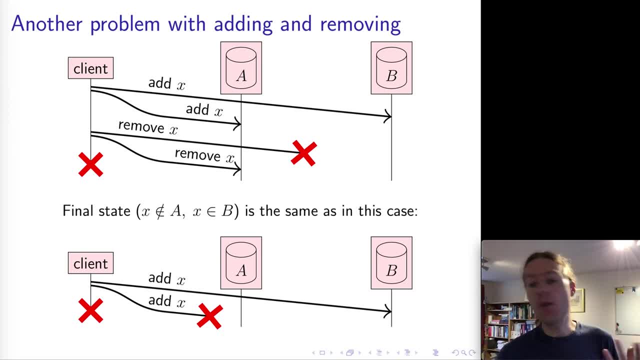 two examples, But actually we don't want it to be the same because the user intention was different In the case of the first scenario. here the user first added, then removed. So the user intention was that the final state should be that x is not in the set, Whereas in the second scenario 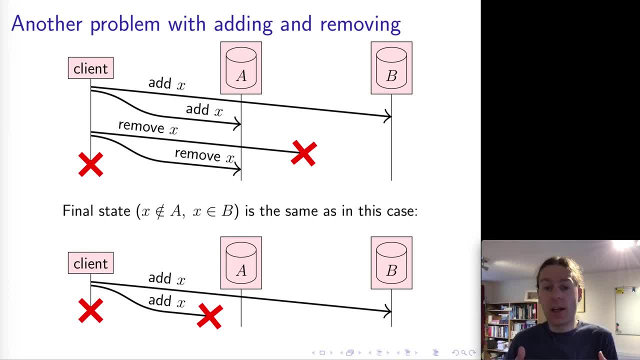 the user only added. the user didn't remove anything. So the user intention is that x is present in the set. So the user intention is actually different in these two, But from the point of view of the replicas these two outcomes look the same, And so we have to distinguish these. 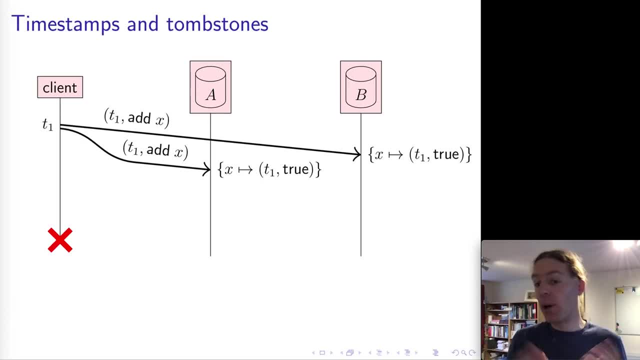 two outcomes, And the way we can do that is by adding timestamps to things. So we're going to reuse what we've learned before about logical timestamps And we're just going to have the client generate a logical timestamp when it makes the request to the two replicas. 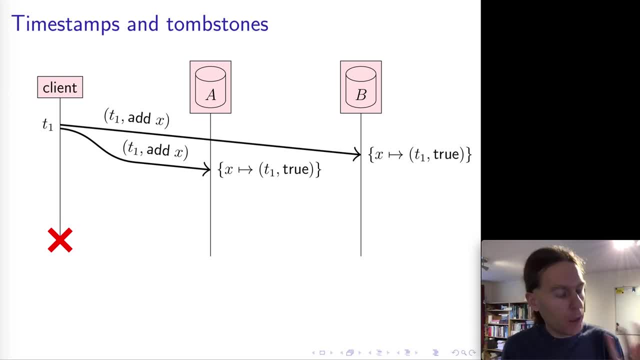 And so the client generates this timestamp t1, and it attaches t1 to the add request that is sent to both A and B, And now A and B both store this timestamp t1.. And I'm also going to associate here x with a value. true And true here just means that x is present in the set And we will see in a. 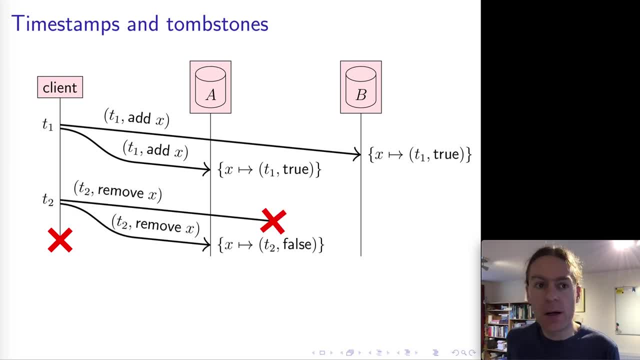 moment why we need this? Because what happens next is now the set is present in the set And the client makes a remove request And because this is a new request, it makes a new logical timestamp t2, attaches t2 to the request. The request is sent to both A and B Now because 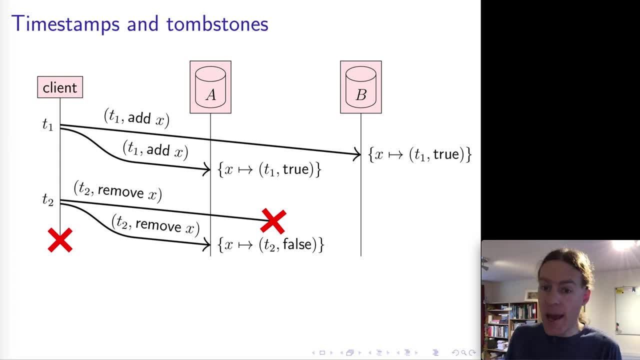 this is a logical timestamp, and the remove happened after the add. this means that t1 will be less than t2,, t2 will be greater than t1. And so here we have replica A receives the request to remove it remove x. And so, instead of actually removing, we're going to remove the request to. 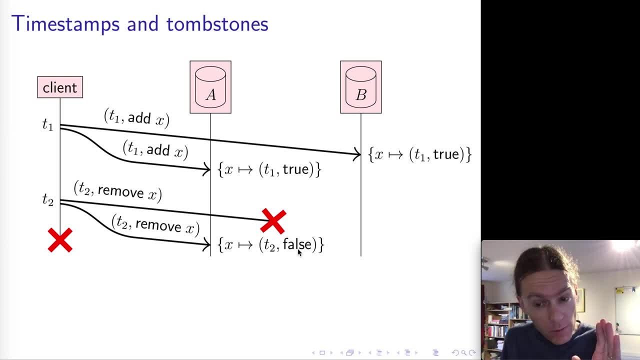 remove x from the database. A leaves x in the database and says actually we're just going to attach this value false here to x, And false means treat the value x, treat the element x as if it were not present in the set, because the user asked that we remove it. But we're not actually. 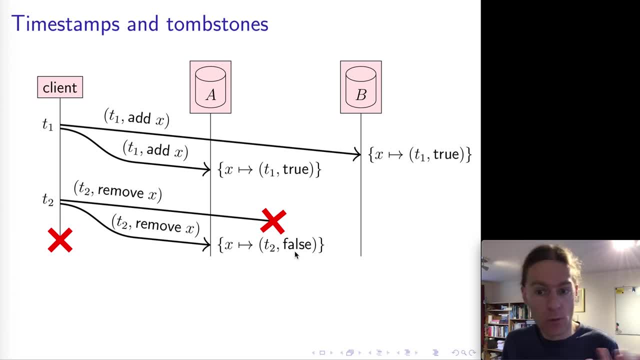 going to remove it because otherwise we wouldn't know whether the user added or removed it. So we're going to leave this marker in the database, marked as false, saying x is not actually in the set And the deletion is going to be false. So we're going to leave this marker in the database. 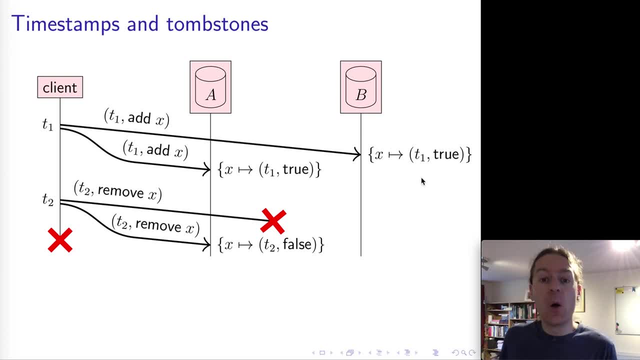 with a timestamp of t2.. So here now we can distinguish. on B, we have that x is present because it has a value of 2, with a timestamp of t1.. On replica A, x is absent because it has a. 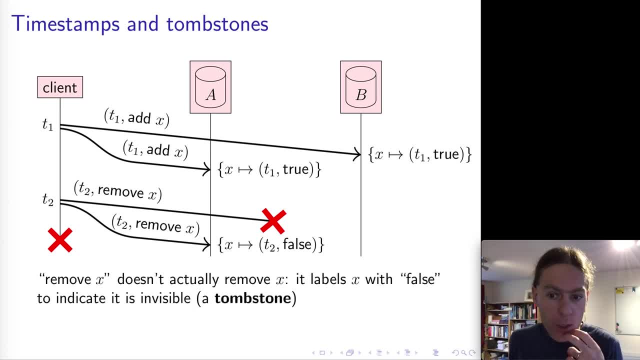 value of false and a timestamp of t2.. So this construction, where we don't actually delete something but just mark something as deleted, is called a tombstone, And this appears in various different distributed algorithms when we have to deal with deletion. So tombstone, just. 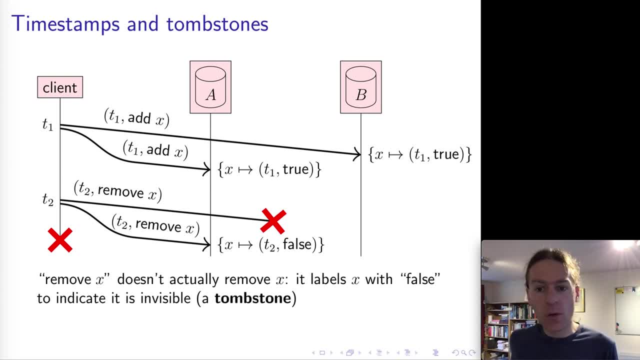 means something was supposed to be deleted, but for internal reasons we had to actually keep it, And maybe tombstones can get garbage collected at some later point in time. that's a separate question, But for now we just need to keep remembering this item, even though it has been. 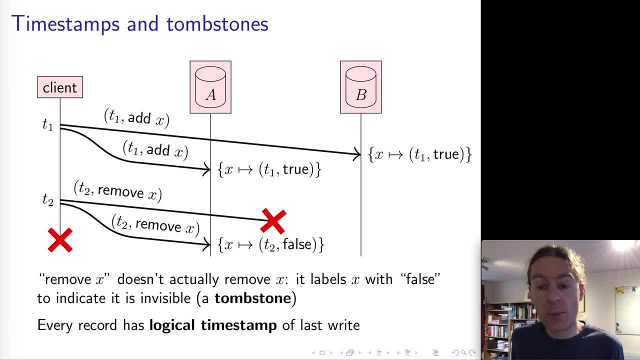 deleted And of course we attach this logical timestamp. So every time some object in the database is written, we attach the timestamp of t2. And of course we have to remember that the last operation that wrote it And this allows us to tell which values are newer and 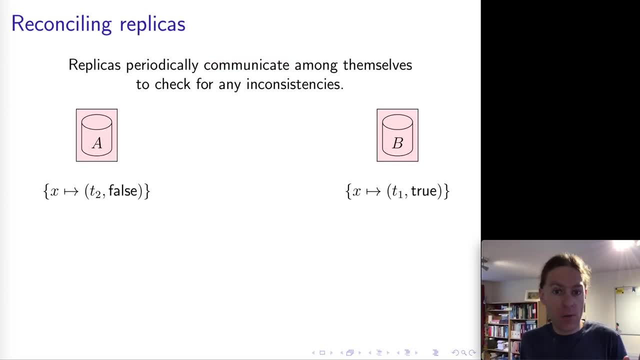 which are older. So this means now that, after this has happened, A and B are no longer in the same state, because A received the request to delete x with a timestamp of t2, whereas B did not receive that request because it got lost in the network, And so, according to B, x is still. 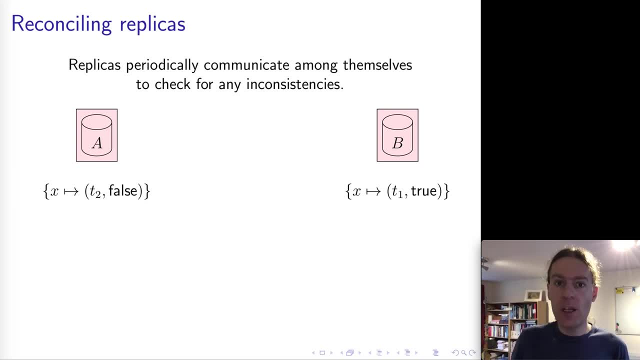 present in the set and it has a last modification timestamp of t1.. And now the two replicas can run a protocol in which they compare what they have, they compare their data, And this protocol is called an anti-entropy protocol, because I guess it's sort of it's supposed to. 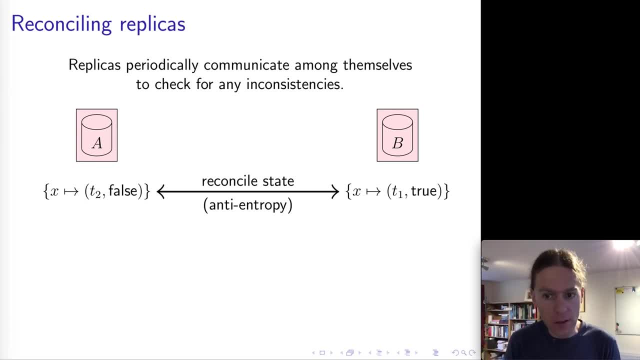 clear the entropy and the confusion and the uncertainty in the system and bring all of the replicas back into the same state. And so, as A and B reconcile their state and perform this anti-entropy protocol, they will compare their timestamps And since we have these logical 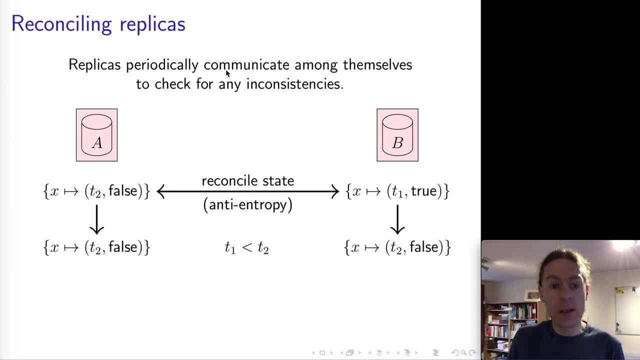 timestamps attached to every data item, they can realize that t1 is less than t2.. So therefore, this value that B has must be older, the value that A has must be newer, And so therefore, the object, the record on B, is going. 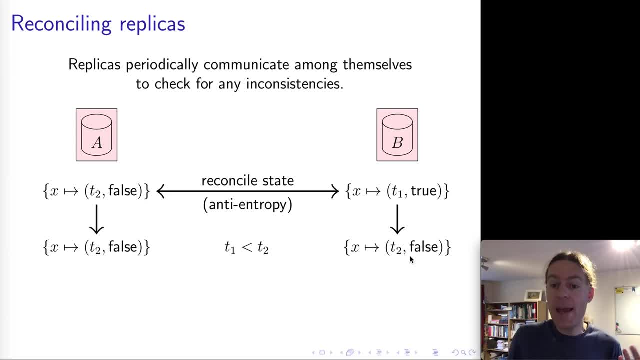 to get replaced with the one from A. So the one from A is the more recent one, so that gets propagated to B. And so here the timestamps have helped us because they tell us about the recency and the relative ordering of these updates. So timestamps have been very 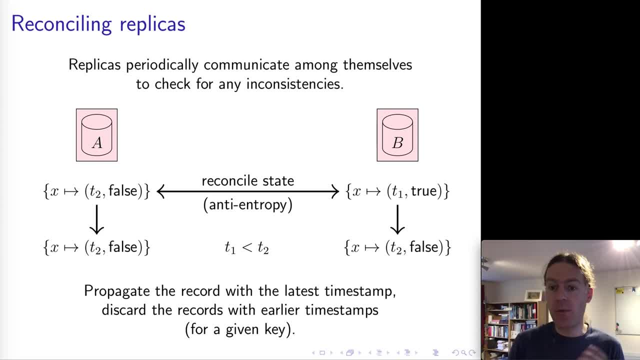 useful. So typically we will probably have one timestamp for every given key or every object in the database, because that's the granularity at which we're going to do that reconciliation. Now, what kind of logical timestamps do we use here? So in our last lecture we saw the 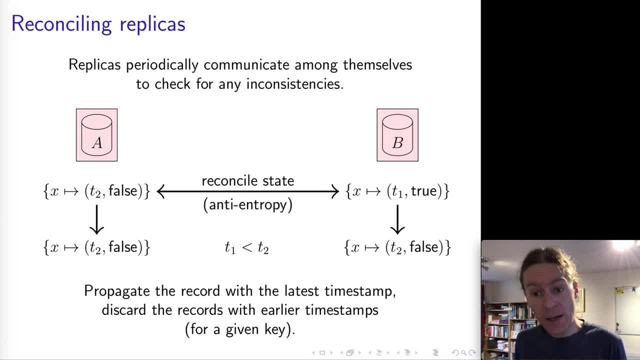 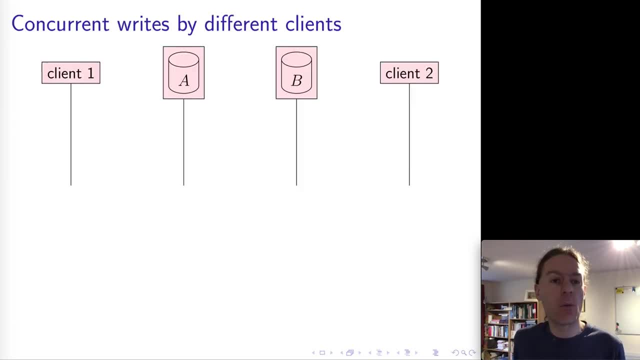 distinction between Lamport clocks and vector clocks And in fact we can use both in databases and we get slightly different behavior. So it really depends what behavior we want, And this becomes apparent if we consider two clients that are making writes to this. 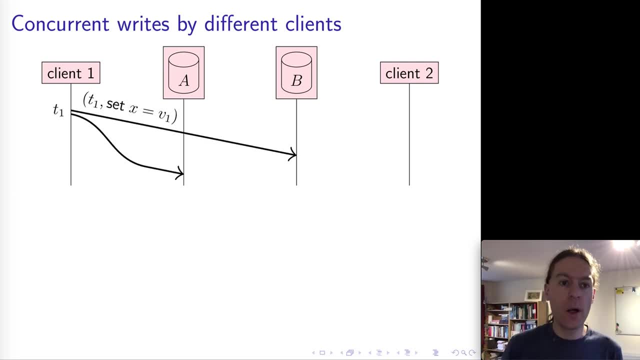 replicated database concurrently. So here on client 1, client 1 wants to update the value that is associated with some key x. So x is the key. v1 is the value that client 1 wants to attach to x, And this operation is going to have a logical timestamp of t1.. Concurrently, while this 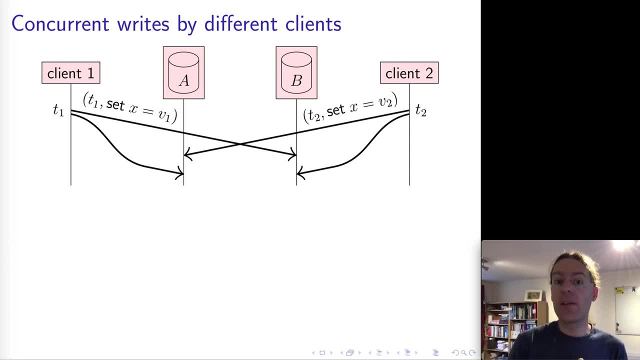 is happening. client 2 also has to update the value that is associated with some key x. So this is going to have a logical timestamp of t2.. And client 1 also wants to set the value of x. It wants to set it to a different value, v2.. So client 1 also generates a logical timestamp, t2,. 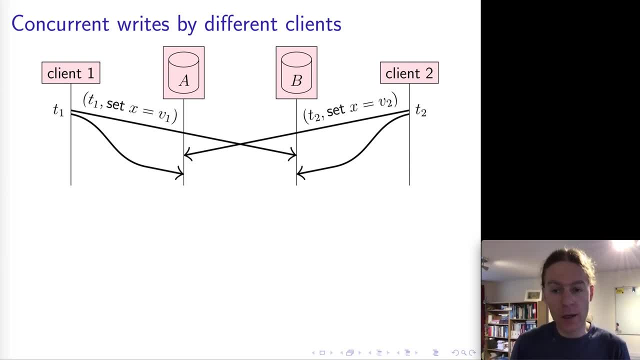 sends an operation of the network attaches t2 to this operation. The operation is: I want to set the key x to the value v2.. Now notice that replica A first receives the request from client 2, second receives the request from client 1, whereas replica B receives them in the opposite order. 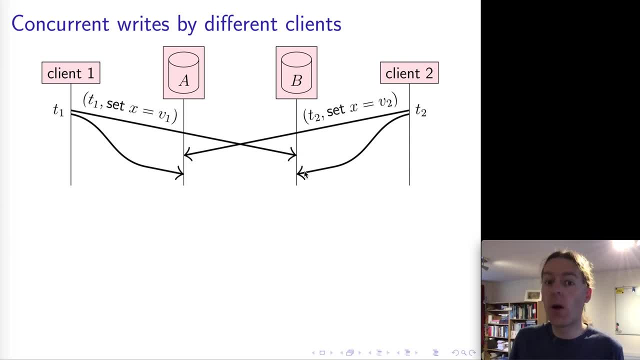 replica B first receives the request from client 1, then the request from client 2.. So this means the replicas can't just use the order in which they see the requests in order to determine whether v1 or v2 is the final value for x. because if they did just use the order in which 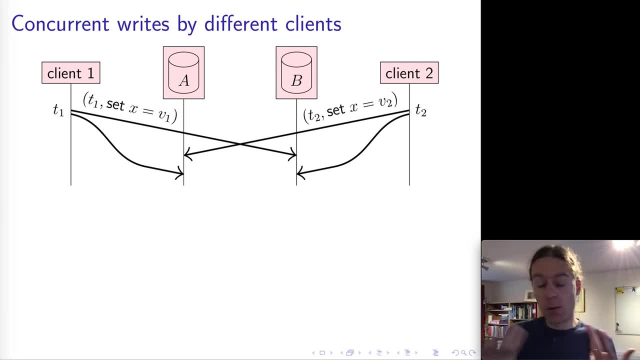 the requests arrive, then they would end up in different states. They would end up inconsistent at the end, And so what we want in a replicated system is that all of the replicas end up being in the same state. Otherwise it's not replication, And that's why we need to use the 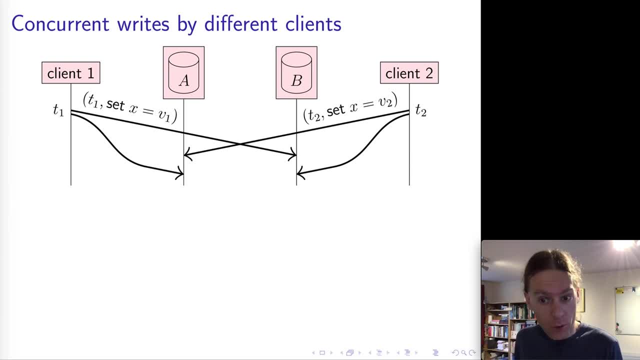 timestamps here, because the timestamps provide a relative ordering of these two operations. Now one option is that we use Lamport clocks, And if you remember what we have with Lamport clocks is they give us a total ordering. So total ordering means that for any two timestamps that 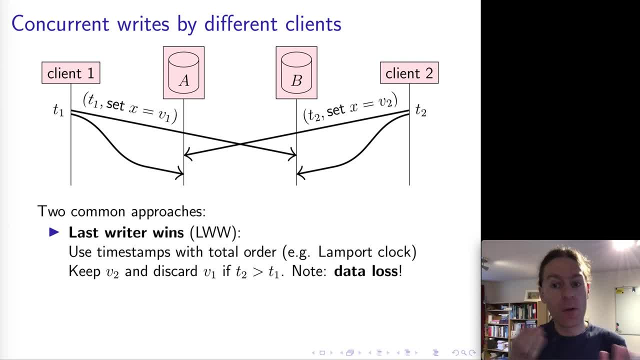 exist in the system, we can always compare them, and it will always be the case that one is less than the other. And so in this case, for example, we can say that t1 is less than t2,, but it might just as well be the other way around, So we can say that t1 is less than t2,, but it might just as 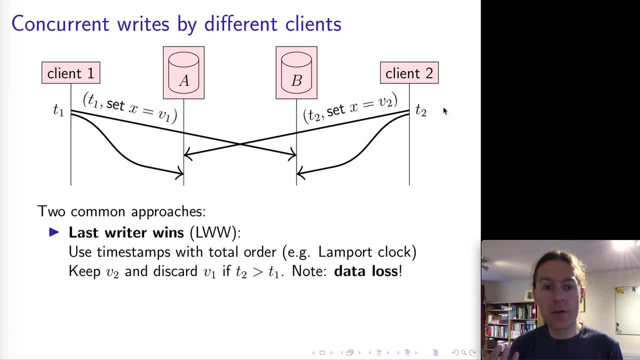 well be the other way around, And so in this case, for example, we can say that t1 is less than t2, because in this case the two operations are concurrent, And so the ordering that the Lamport timestamps provide us is arbitrary, essentially. And so what we can do here, 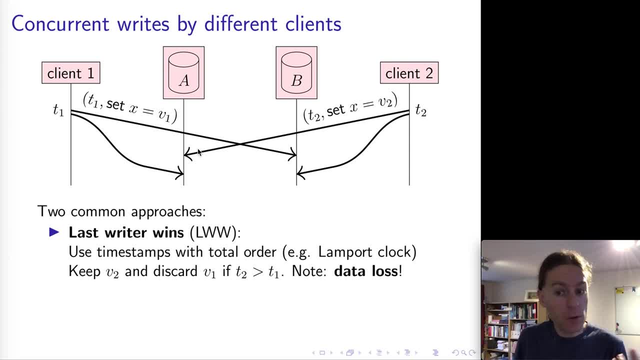 for example, is that we compare t1 and t2, and we just keep the value with the higher timestamp, And this will work, because then, as the value gets overwritten, we know that the overwrite happens after a previous operation and therefore it will always have a greater. 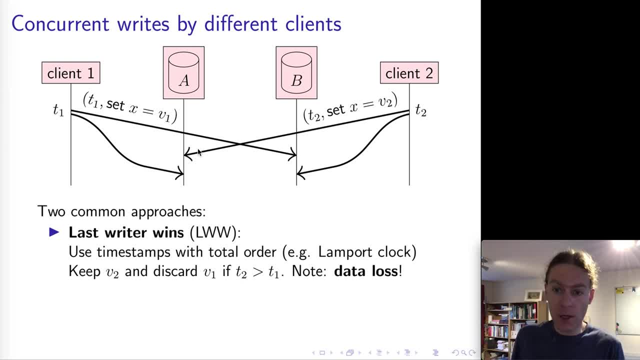 time stamp, And so we can say that t1 and t2 are concurrent and we just keep the value with the timestamp. So therefore, overwriting a smaller timestamp with a greater timestamp is a fine thing. You can do that, And this behavior is called last writer wins, because we assume that. 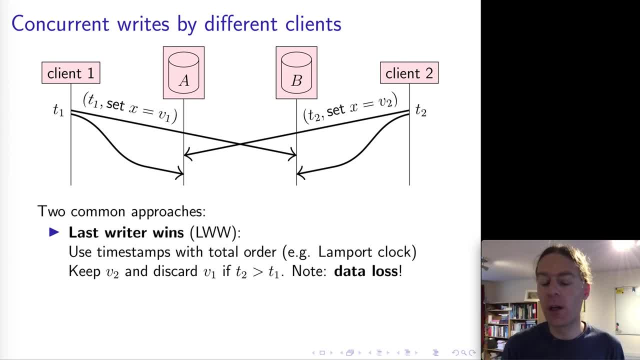 the last one. the last writer is the one with the highest timestamp, And so the highest timestamp wins if there are several concurrent updates with different timestamps. Note, however, that this means that if, say, t2 is greater than t1, this means we keep v2, which was written by client 2,. 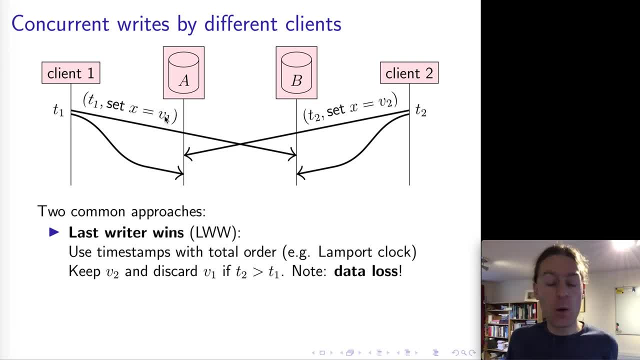 and we simply discard v1.. So value v1 is simply gone. So we're not even storing that value anywhere. It simply gets overwritten and forgotten. And this might be okay, depending on the application. There might be applications in which, actually, if there are two concurrent writes, it's fine to just keep one. 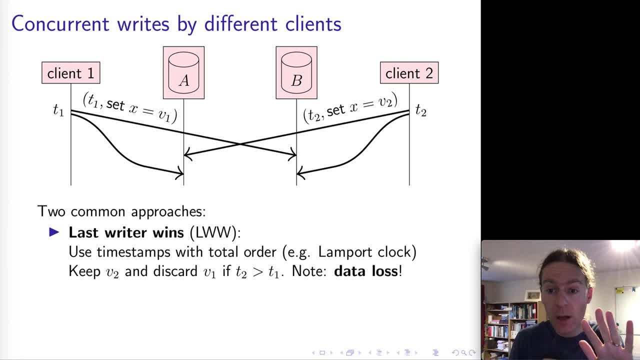 and throw away the others. If there are five concurrent writes, we're going to keep one and throw away four of them. But there might also be scenarios in which, actually, if there are several concurrent writes, we want to keep all of them and we want to explain them to the client. So 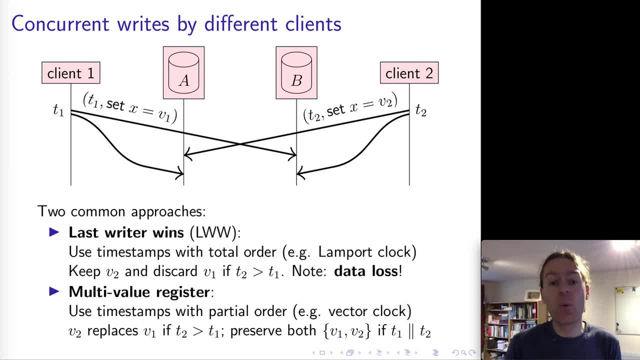 we can explicitly resolve this situation And if we want that well, we use a vector clock instead of a Lamport clock. If we use a vector clock, then if we generate two different timestamps- t1 and t2, and these two operations are concurrent, then the vector clocks will also be. 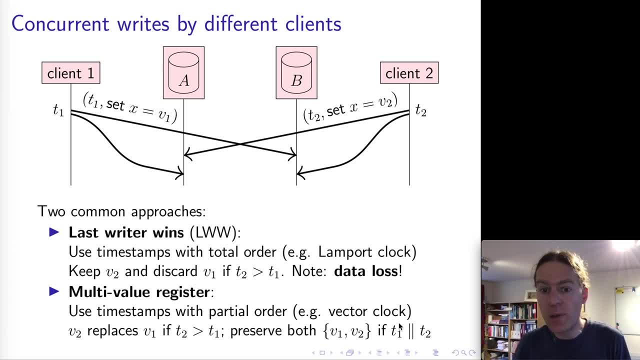 incomparable, We will end up with t1 and t2 being incomparable, And this allows us to detect the fact that these two operations are concurrent, And so in this case now, we will only overwrite one with another value if their vector timestamps are the later one strictly greater than the earlier. 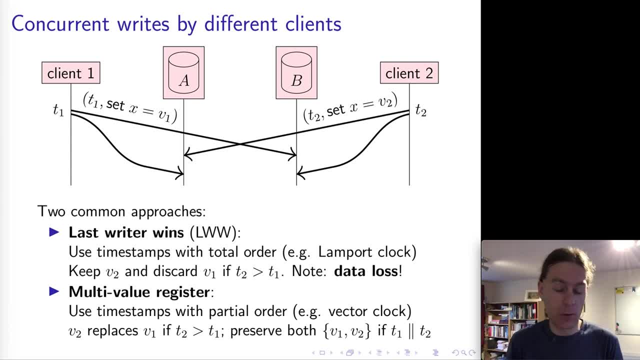 one under the strictly greater than relation that we've defined previously. But if we have two concurrent updates, then we will keep both of them, And so in this case now there's not a single value attached to the key x, but there could be multiple values, in this case v1 and v2..